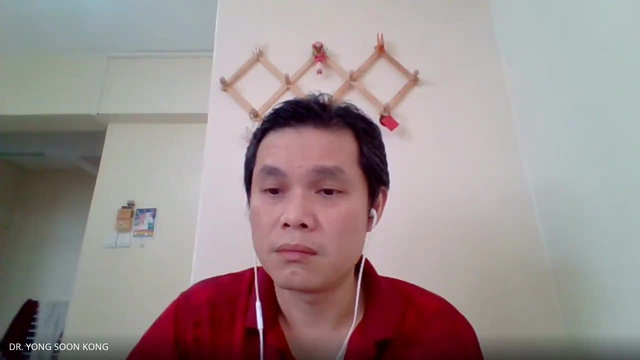 Seriously, I don't know why is the setting wants somebody to let it in, because I never received anything to like enable people to join. Seriously, I don't. I guess they have to follow the YouTube video later on, unfortunately. So, people, I think I cannot wait any longer. I will just start with the lesson. 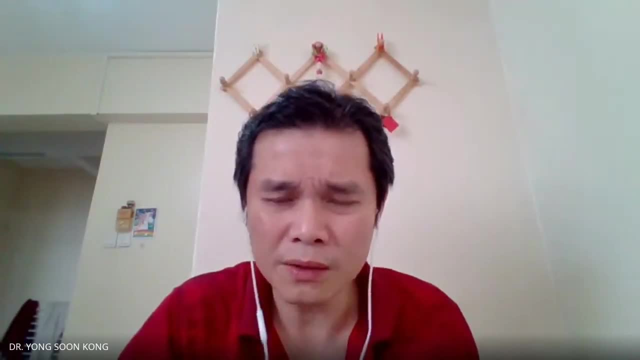 And then the rest of it who cannot join. maybe you can join the YouTube video later on, So don't worry, We're going to come back to that later on. I'm going to start with the next lesson, which is about soil acidity. 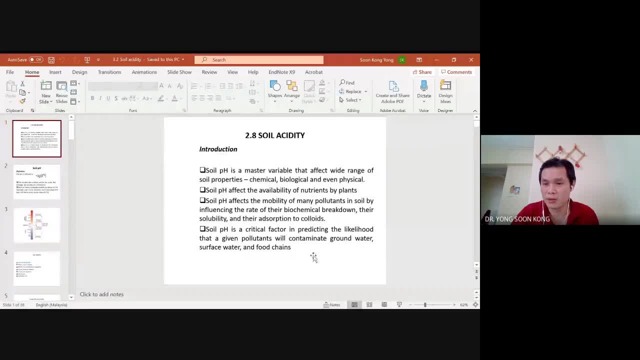 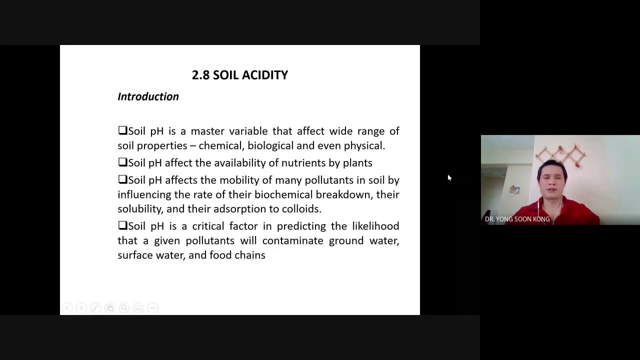 Now, in essence, this lecture will be talking about how soil pH affects the usability of the soil. So it's not just for agriculture, It's for everything, Because when it comes to pollution and its effect to human and also agriculture, pH can be said to be the major source or the major factor that can determine whether that soil is good or is bad. 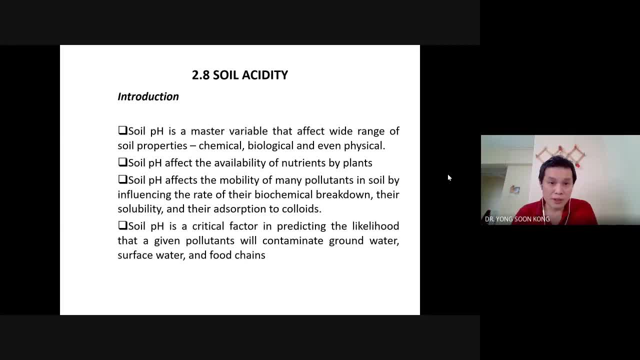 pH alone, seriously. Okay, Now for introduction. I think pH don't need. I don't need to introduce to you what is pH and what are the everything. By the way, this slide actually, This slide actually is the main points of the details that we're going to go into. 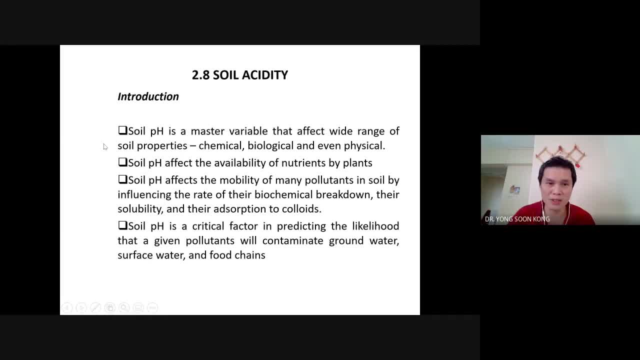 So before I go into the details, so what pH is so important? because it actually can determine a wide variety of chemicals And in essence, it also affects other parameters. So soil also. soil pH can determine whether a nutrient can be absorbed by plants or not. 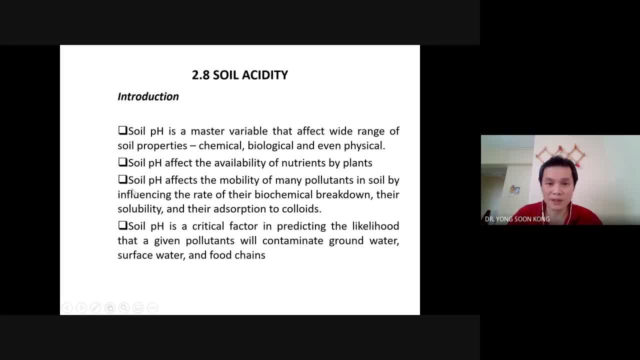 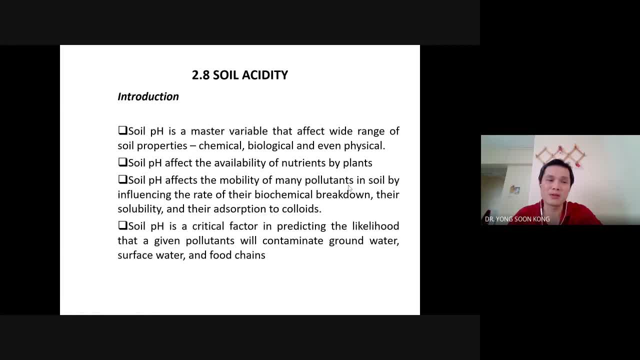 to human, because a soil can be said to contain heavy metals, but at some pH these heavy metals is not dangerous to human. So don't think that the soil will have toxic heavy metals. They always need to be treated. No, not. not necessarily, because if there are certain suitable pH, these heavy metal 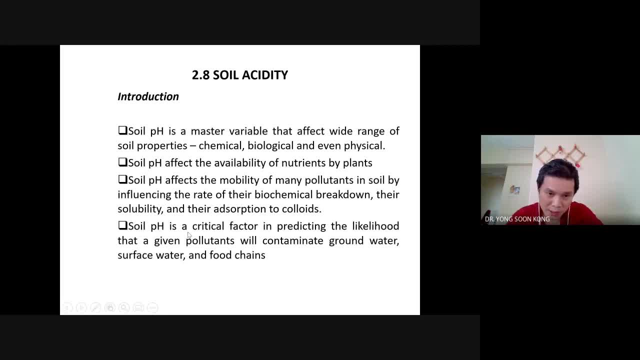 will not harm people. yeah, and then last point: soil ph is a critical factor in predicting the likelihood that given pollutants will contaminate groundwater, surface water and food chain. so there you go again. at certain ph, some heavy metals might comes up in your groundwater and this is how they. 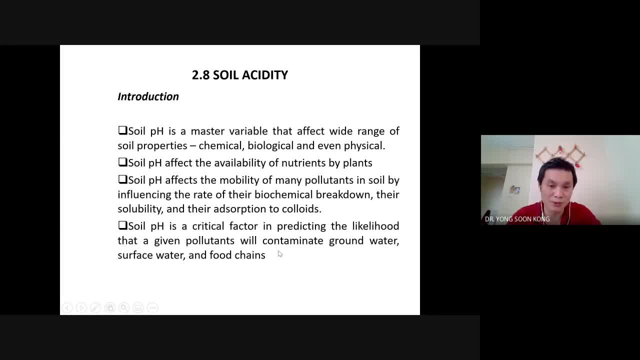 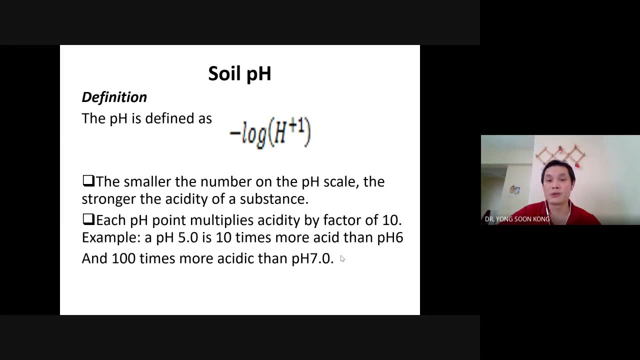 harm human if people consumes it and also if it is a wrong ph, this heavy metal might go into the food chain, not further ado. it's like now this one i think i can skip already again, because this one i believe you have seen it before in secondary school, so i will skip now probably. here i'm going. 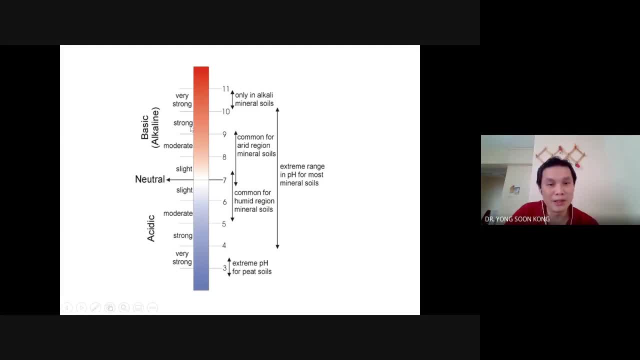 to stop for a while and explain to you what is the ph range. so basically neutral ph is seven. everybody agrees on that one. anything higher than seven is considered alkaline. so the higher it is, the more extreme the alkalinity. so if it's nearer to 11 it says to be very strong basic or very strong alkaline. i haven't seen any soil that reach beyond 11, but i leave. i believe there is because limestone soil soil that majority of the limestone can be as high as 14, so i believe this one is as high as 14, imagine, and also it goes to the. 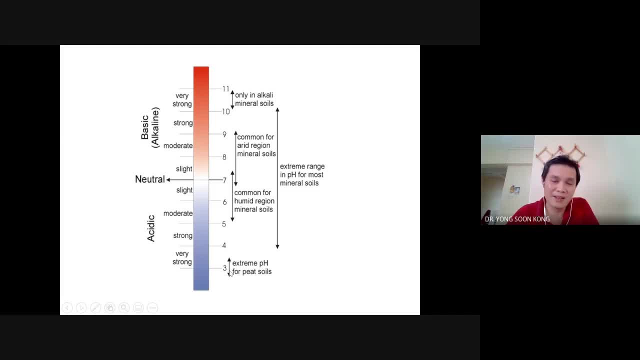 opposite end. now, any ph less than seven is said to be acidic. it could be up to three and, believe it or not, some of the soil samples can reach as low as one or maybe even minus. oh, by the way, the strong acid that you use in the lab, like, for example, your sulfuric acid or nitric acid, when you measure the ph, don't be surprised: the ph isn't that strong as aポ. 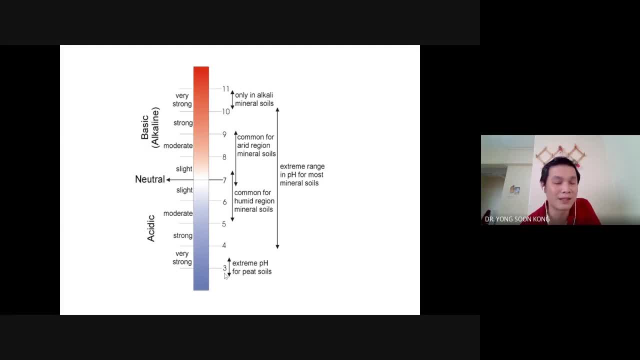 pH value can get to negative. one negative something, Yeah, it can be that strong acid, But in nature, naturally these are the normal pH that you can see right here. So it depends on what conditions that cause soil to be acidic or alkaline. 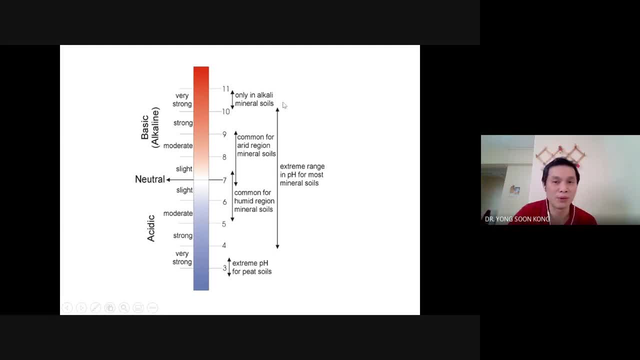 If you have more limestone, automatically it becomes more alkaline. I think beyond that not many soils can be alkaline. So usually alkaline soil are those from arid region. Arid means dry and hot, like the deserts. Desert is said to be arid region. 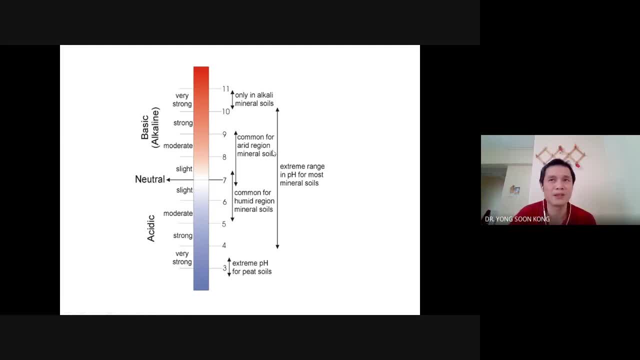 So usually they are going to accumulate a fair bit of earth- alkaline metals- So that's why they're alkaline. However, on the other side, on the other end, if it's more acidic, like here, it is mostly due to the presence. 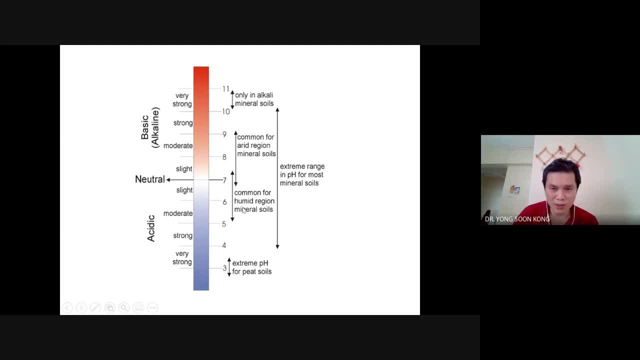 of organic matter, See Humid region, mineral soil, and then, if you are very, extremely acidic, it has peat soil. Now, the presence of organic materials alone, if you say just organic material, they themselves is not very acidic. Now the very reason. 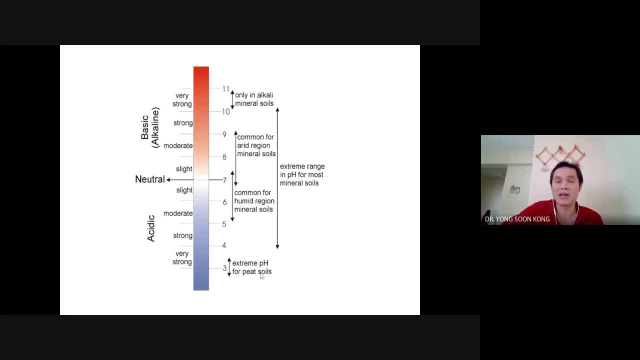 why peat soil is acidic is due to microbial activity. After this I'm going to explain more to you why peat soil. they are very acidic. But of course there is one more factor that is not included here. That is: 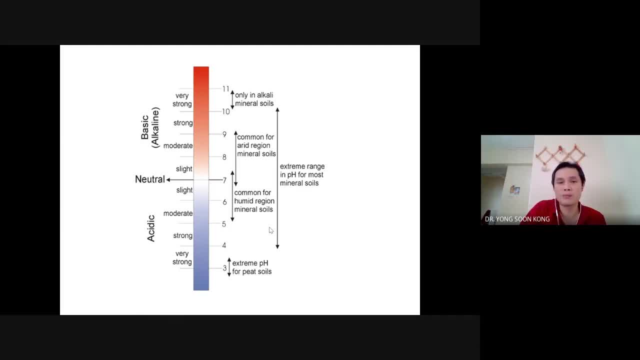 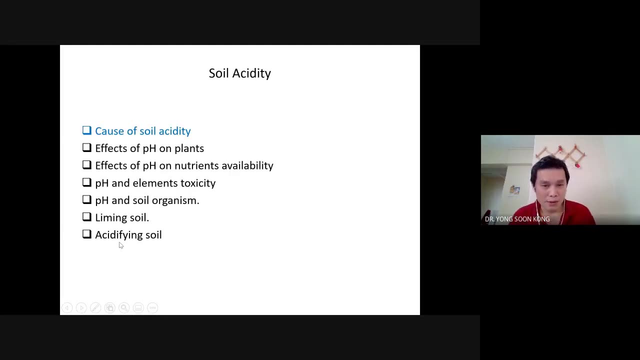 I think you should know also the anthropogenic pollution. Anthropogenic pollution also cause the majority of acidification of soil, in which I will also explain to you later. So this is the outline of the content that we're going to talk about. 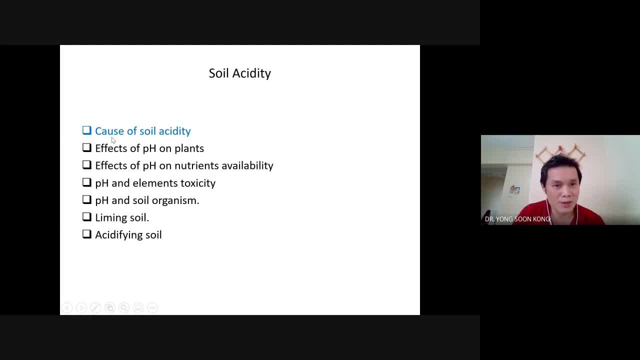 So this is the outline of the content that we're going to talk about. So this is the outline of the content that we're going to talk about. We're going to learn, for the next, hopefully, 30 minutes, the cause of soil acidity effects to plants. 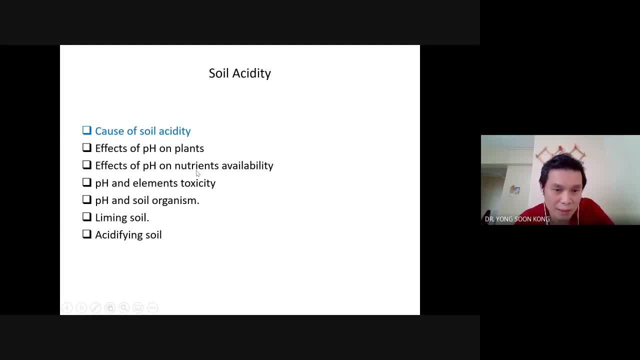 effects to soil pH and its nutrient availability and how to solve this problem. But of course, in between we're going to explain how pH becomes acidic and how pH becomes alkaline. Okay, now we're going to begin with the cause of soil acidity. So earlier, 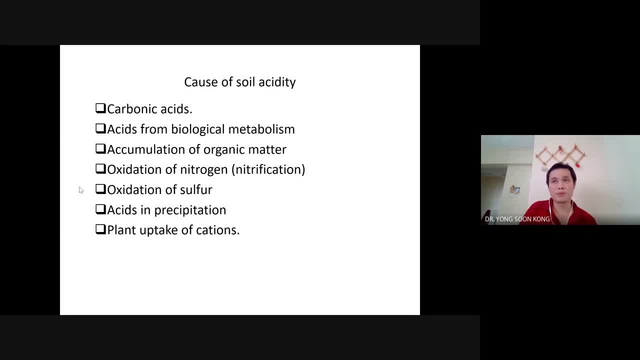 I've told you peat soil is acidic due to microbial activity, but there are actually many. so the first, the first one: carbonic acid. i'm sure you've learned this is from grey water. naturally it contains rain. uh, natural rain contains carbonic acid. i'll explain later how. 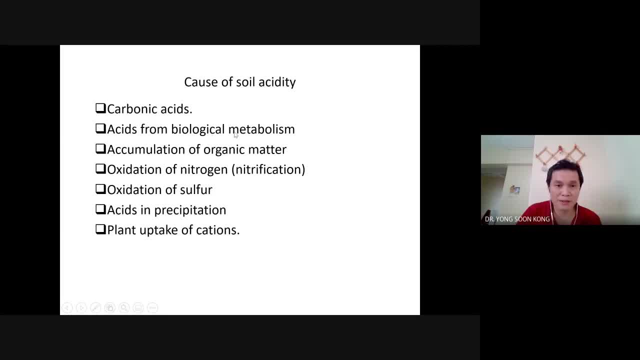 uh. so microbial metabolism, microbial activity, activity, as well as the accumulation of organic matter, these two actually comes hand in hand. they come, they come in together. whenever you can find organic matter, you will find metabolic uh, biological metabolism, and together they contribute to acidic soil. however, there are other factors as well: oxidation of nitrogen. 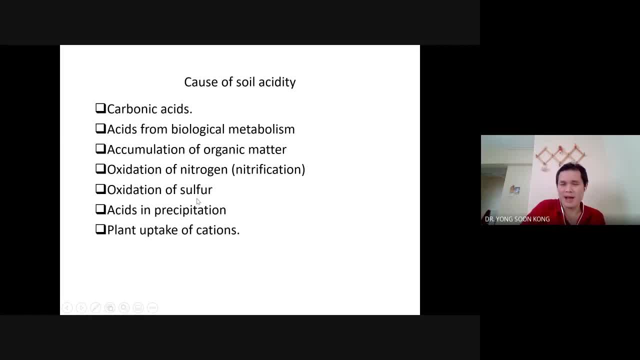 oxidation of sulfur. remember just now i said anthropogenic pollution. ah, this is. these are the two: oxidation of nitrogen and sulfur. again, i'll explain to you more about that. and because of this one, they mix with rain water and it becomes ac, a precipitation and plant uptake. 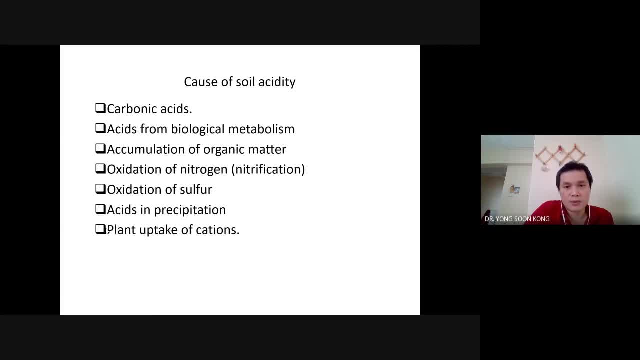 so, basically, there are three factors, i would say, two of which is natural. one is due to man-made oxidation of nitrogen, sulfur and acid precipitation. these three, right here they are circling, they're actually man-made, they're, they're actually caused by anthropogenic solution. uh, pollution, the rest of it is naturally occurring. yeah, i'm saying about carbonic acid. 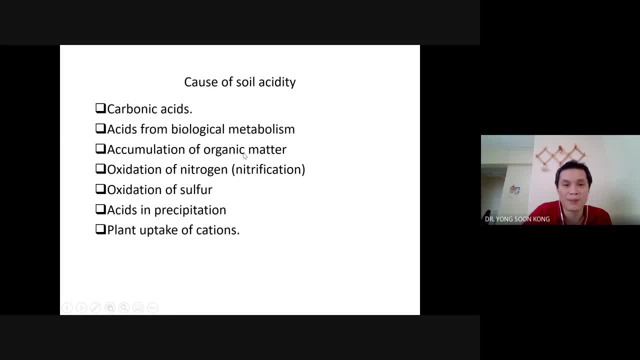 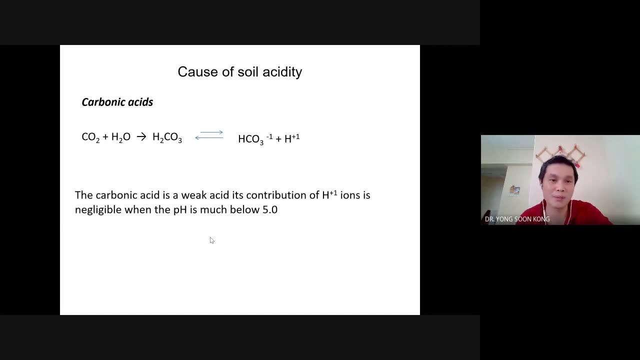 acid in biological metabolism, accumulation of organic matter and plant uptake- these happen naturally, yeah, so don't you worry if you don't get what i said just now, because now i'm going to explain to you one by one. so i'm going to start with carbonic acid now. 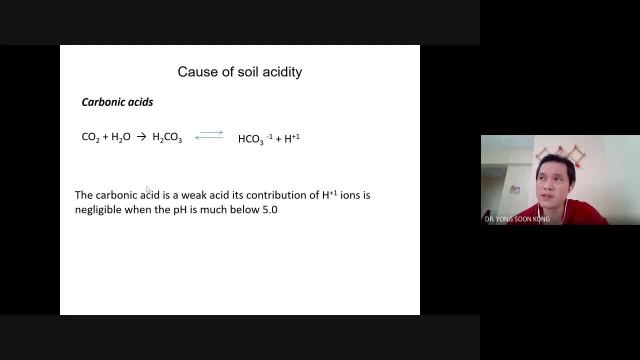 natural rain, natural precipitation. if you see the first instance of rain after a long period of drow- so after several days of no rain- suddenly you have one ring. if you manage to collect the rain water, it may have a little bit of carbonic acid and it's normal to have rain ph around five. 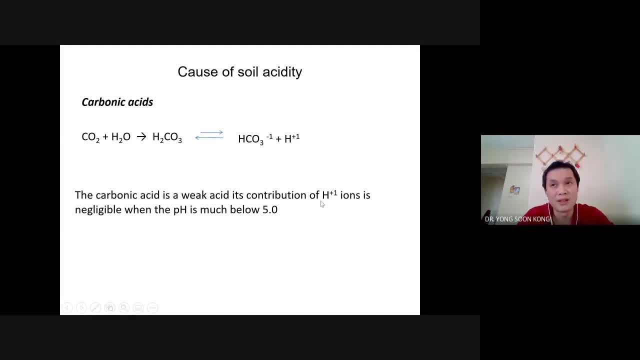 four point five, five point five. that is natural, actually, but sometimes you may find out that this rain ph- if it's raining too heavily, it comes back, comes back to seven. so it fluctuates a lot depending on how much of carbon dioxide that you have, because carbonic acid, as you can see right, 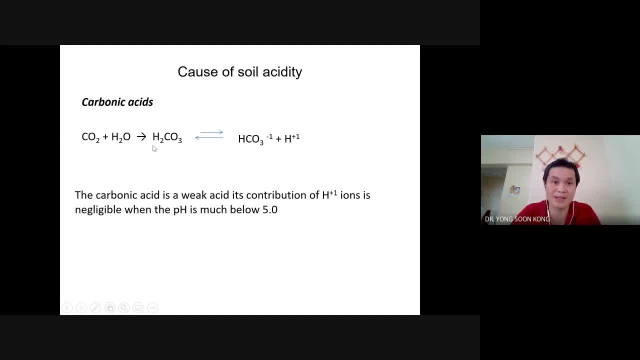 here h2co3, this is the carbonic acid, is produced by the interaction between carbon dioxide and water, and they will become acid when they dissociate. so this uh, two directional arrow, as you can see right here, is the dissociation where they produce one hydronium h plus. so this is the acid, yeah, this one that caused the acidity of soil. 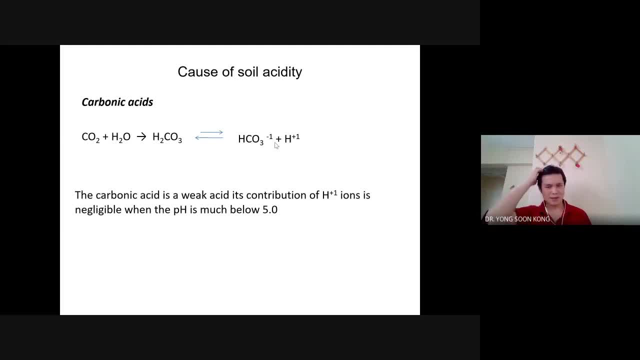 and uh, when you, when you go to like places like guatapuro, guernia, you have stalactite and stalagmite. how does calcium carbonate are being sort of dissolved. uh, this is how they dissolve. they dissolve due to the presence of carbonic acid. 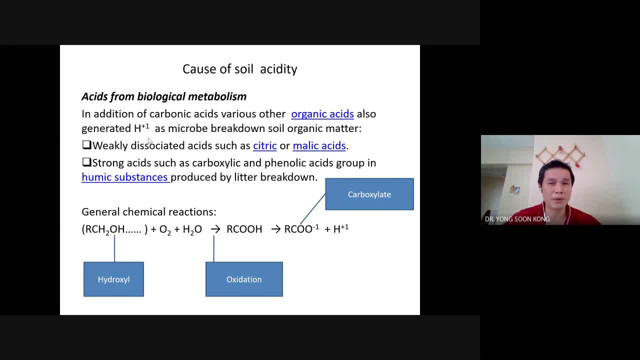 okay, moving on to the next one, acid from bio biological metabolism. so i think i'm going to discuss, together with the next one, accumulation of organic matter. yeah, but first thing first. microbial activity or biological metabolism can only arise if there are presence of organic matter or, in this case, it comes from. 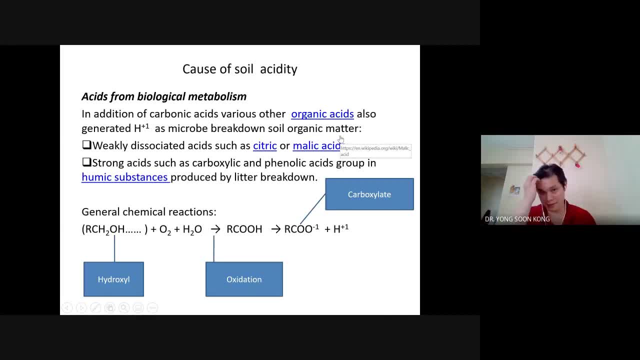 the breakdown of soil organic matter. now, as you know that this organic matter can be from plants, can be from um from animals, now, as long as microbes go and breaks them down, they will produce organic acid. now i won't going to click here. you can actually click it yourself and find out what. 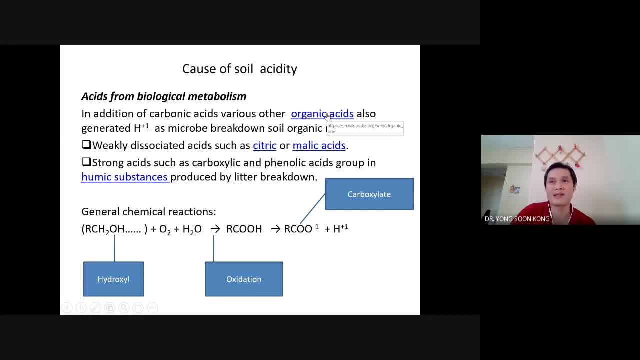 are those organic acid? so when i say organic acid, they contains primarily carbon, a lot of carbons. and what are the functional groups that give some acid? as you can see right here, functional groups such as carboxylic acid, and i think that is it now. sometimes people say hydroxyl is acidic. 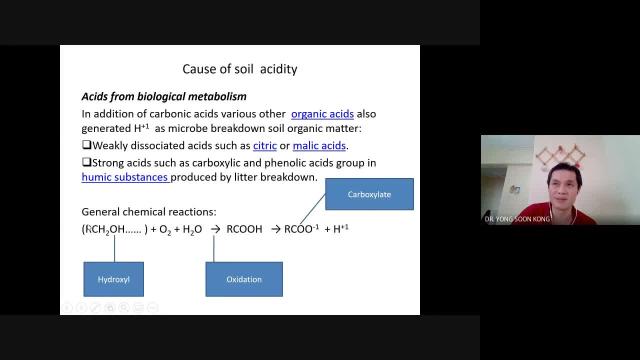 technically, yes, hydroxyl can be an acid, but why do you always hear carboxylic acid? because this one dissociate readily to give you the hydroneph like this one, whereas hydroxyl they don't give you this h plus so so easily. they don't, they cannot break this and they cannot give this one. 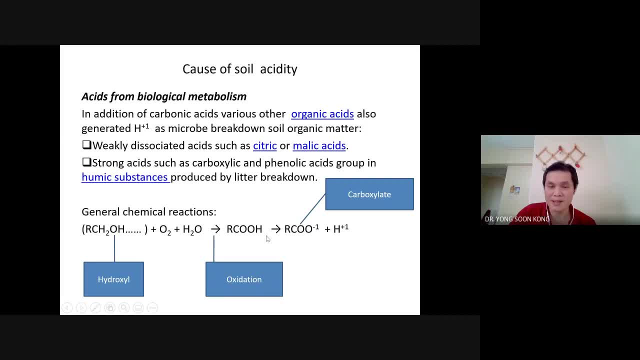 hydroxyl will only become carboxylic acid after this reaction and it's called oxidation, so i put this one arrow here- means oxidation after oxidation of hydroxyl group. then only it becomes carboxylic acid and therefore it gives you the acidity and 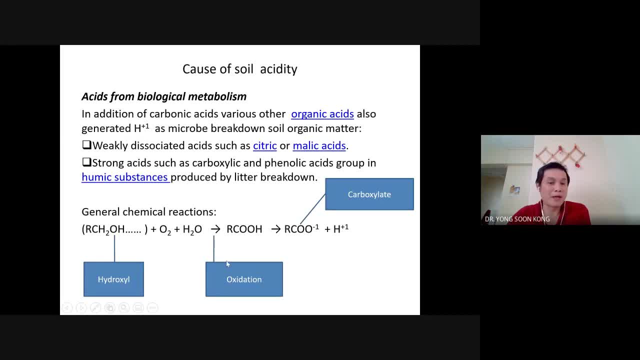 this oxidation usually is due to microbe. microbe does this job. so i think that one clarifies everything. it comes from organic matter and due to microbial oxidation they break down and then they oxidize it. they give you this carboxylic acid and one of the 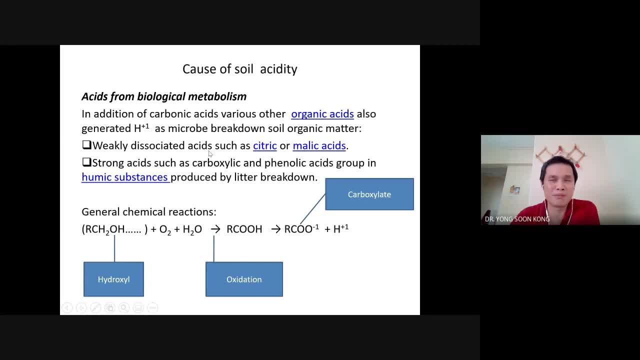 common common organic acids that produce from microbial metabolism includes citric acid. this one, you can find out how it looks like. you have three carboxylic acid group or maybe malic acid. so yeah, if you want to know the structure caricative, click it yourself and then you can know it yourself. yeah, now the other thing that also can. 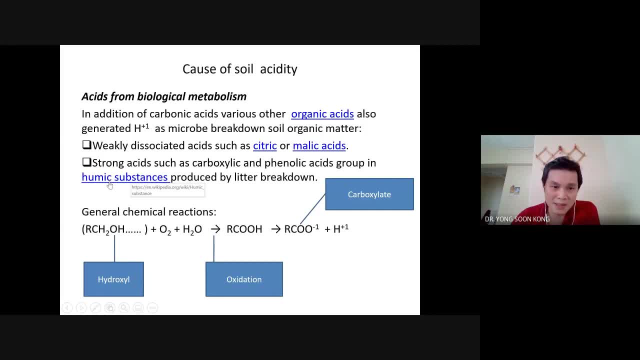 give you a little bit of acidity is humic substance. you see, this one is essentially a soil organic matter. have you heard humus before? yeah, humic acid is the scientific name for humus. humus that you can see, the dark organic matter in the soil. yeah, this is how they look like. 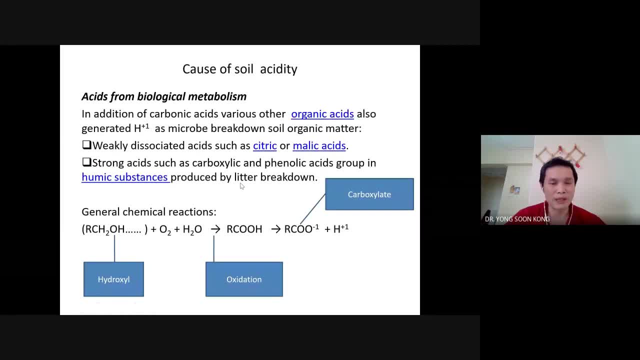 now the structure is very complicated but with the click of this button, with this link, it brings you to wikipedia and you can see how complicated they are. again, they are majority of them hydrocarbon carbons. they have a fair bit of hexagon ring, benzene ring and with that benzene. 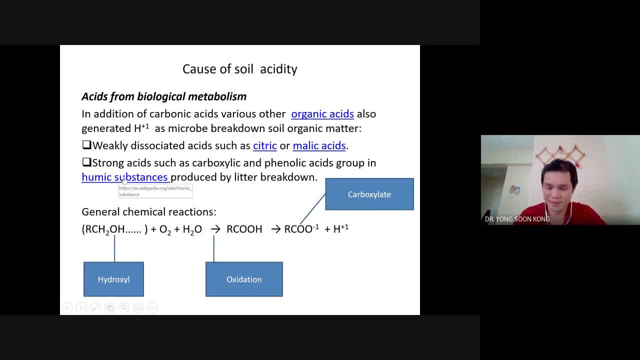 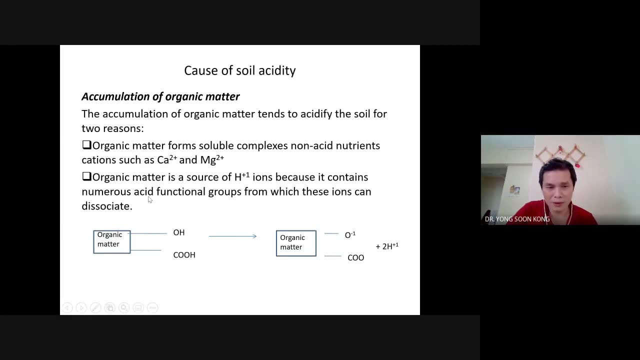 it actually gives a stronger acid. yeah, i'm not in favor of teaching you chemistry, because i know chemistry can take a long time to understand that, so i think i'll just move on to the organic matter accumulation of organic matter now, following on the humic acid that i've explained. 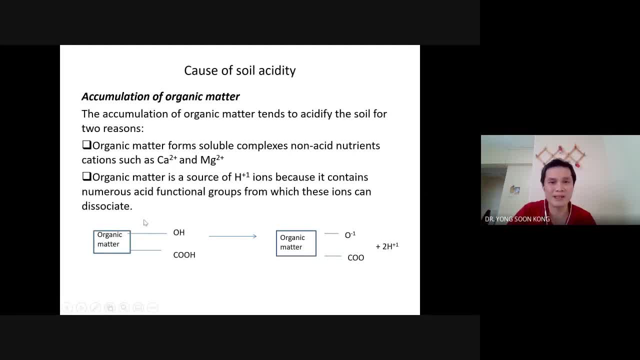 to you earlier why this humic acid is considered acidic. now, that is because the organic matter have these two functional groups, either hydroxyl or carboxylic acid. now these two cannot be acidic. it won't become acidic unless this happened. so once again, from left to right, this reaction. 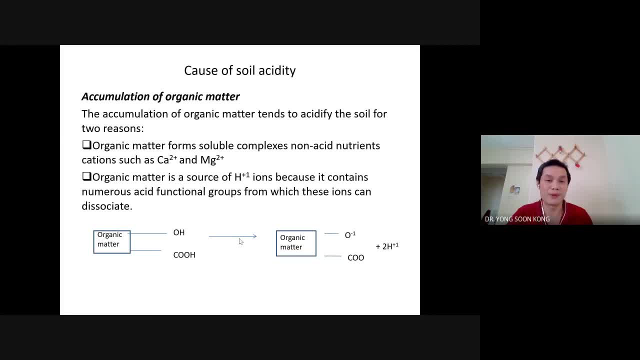 is called dissociation. where is dissociated h plus, h plus dissociated from carboxyl group. h plus also can be as dissociated from hydroxyl. now, earlier i said to you that it's quite impossible to have this reaction from oh to o minus n. 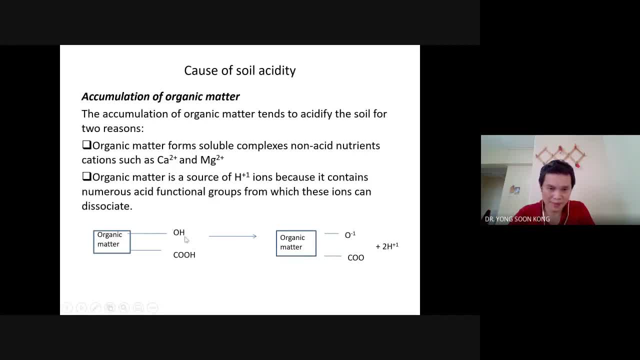 well, that is possible. if this, oh is attached to a benzene ring. yeah, if it's attached to a benzene ring, this can happen. however, is if it's attached to any, uh any- hydrocarbon, long hydrocarbon, it's not going to happen. yeah, long story short. uh, that is organic chemistry. i am not teaching. 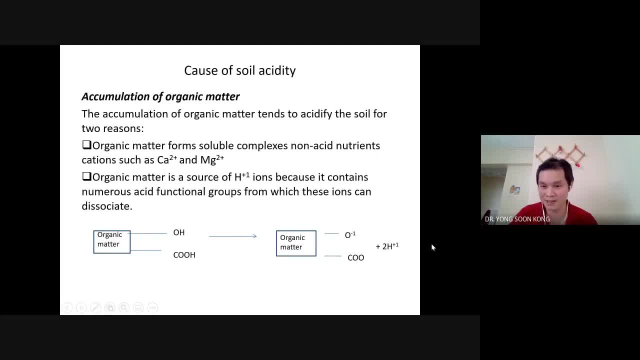 you organic chemistry, so i'm just telling you that you have organic matter, this will happen, okay. and how does this? further brings down the soil acidity by forming this complex. so when you have this negative charge on the surface, it can actually binds with the positive cations, such as 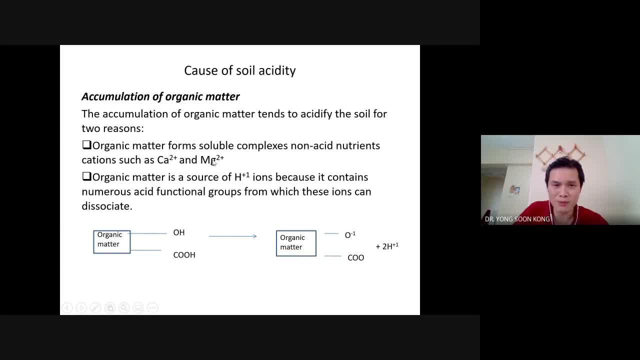 calcium, calcium 2 plus or magnesium 2 plus. now you must be wondering how come bonding between these two cations will further brings down the acidity. now for your information, these two cations are earth, alkaline metal, so which means if these two are present in the soil, the soil becomes. 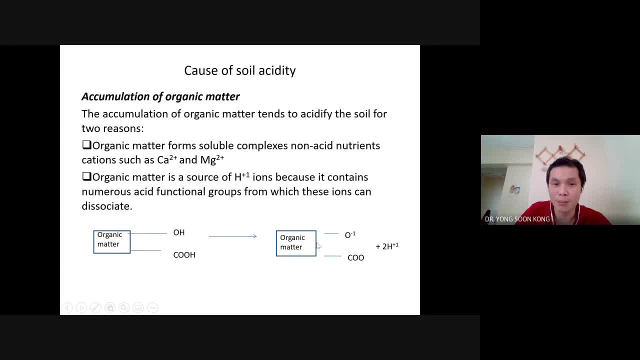 alkaline. however, if organic matter binds with these two cation, it will going to acidify the soil. that means they can no longer mix the soil alkaline. okay, so this is part of the well, one of the reasons why peat soil. they are so acidic because they trap those. 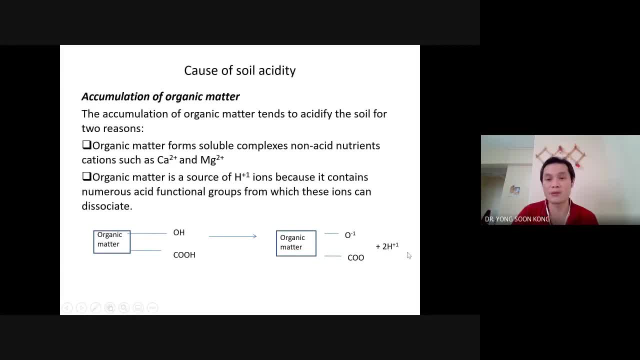 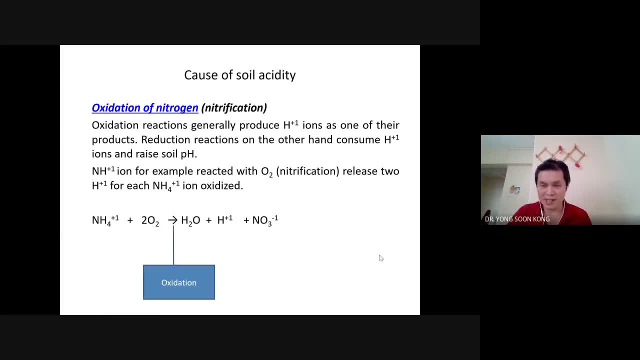 alkaline metals, and then they also, at the same time, can release the acid which is h plus over here. okay, moving on, i think this was quite easy. i believe you learned this before, so i'm not going to talk too much. what i can say is that this one- previously you must have claimed this oxidation. 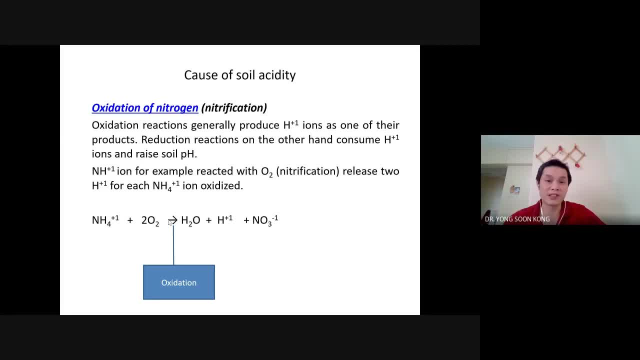 of nitrogen from combustion of fossil fuel. yeah, that is i. i remember exactly because i i thought before diploma. they always blame on the oxidation of the combustion of fossil fuel, because when, when we have a combustion engine and we burn fossil fuel, our air actually contains 70. 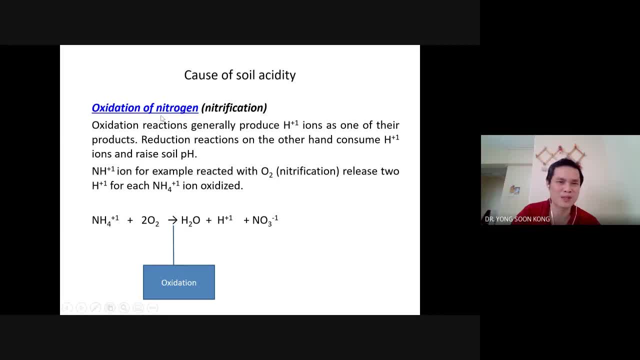 around 70 percent of nitrogen gas, and when they burn it becomes nitrogen oxide, and that is when it becomes- and therefore it becomes this one, the nitric acid. now, what i'm going to tell you more is that actually, agriculture also can cause this one. the way they have this reaction is quite different. it's not through combustion. 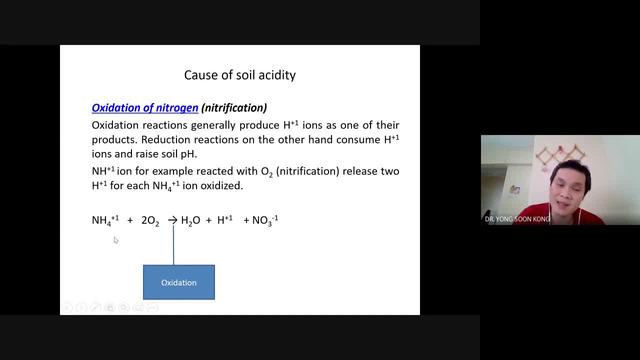 it's by putting in fertilizer. see this ammonium. yeah, this one comes from the fertilizer. this ammonium, when you put it in fertilizer, it does not stay ammonium forever, because we have oxygen in the air and these two reacts regularly. so this one is quite naturally. 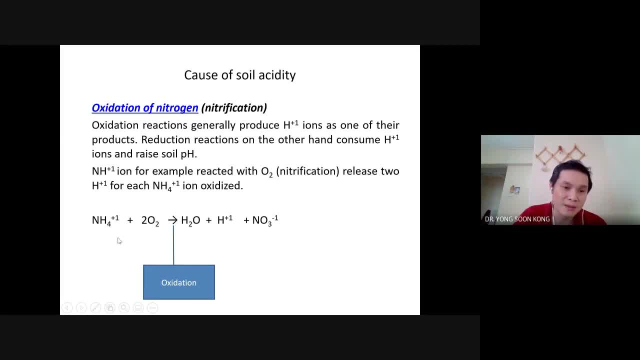 happen because we have oxygen in the air and these two react regularly, so this one is quite naturally happen. the ammonium in the fertilizer will be oxidized by the atmosphere- our atmosphere that we're having right now- and they themselves become nitric acid. and guess what? this is actually the major. 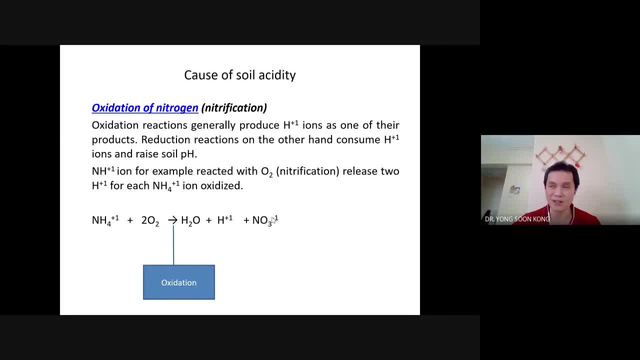 problem in oil palm. mistake if anybody here kampung at felda, you probably have some waterways near oil palm estate. they have like blue, green color and so on. one of the one of the contributors of the bad water quality in these waterways is this one. 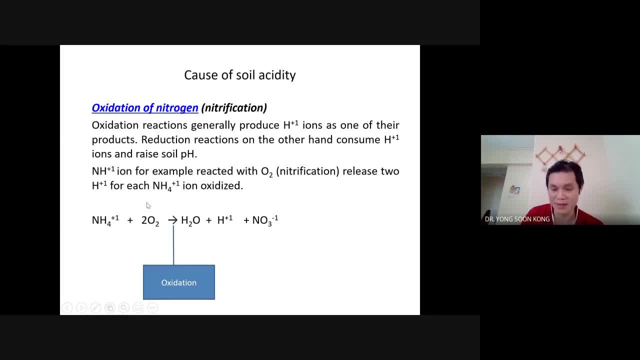 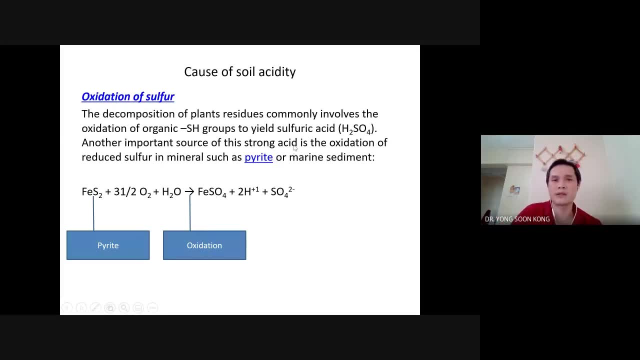 oxidation and acidification of water by simply putting fertilizer- okay. next one is oxidation of sulfur. okay, now, this one is clear cut from the soil itself. while earlier the oxidation of nitrogen comes from fertilizer, this one probably a little bit different. now Sometimes farmers also use a little bit of sulphur in the soil, because sometimes the 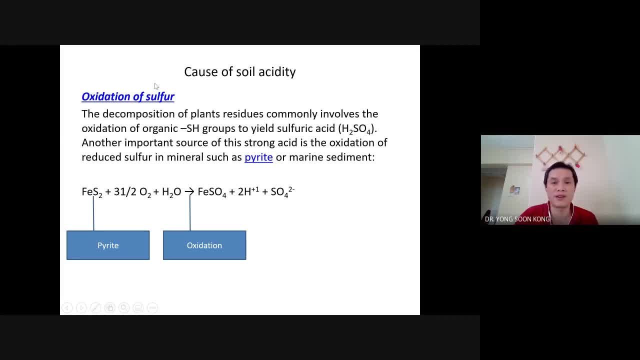 soil may not have the good pH. putting in sulphur acidifies it, But the way they work is quite similar. What is needed here is anything that contains sulphur, Now in this case iron sulphide, or in other words we call it pyrite. 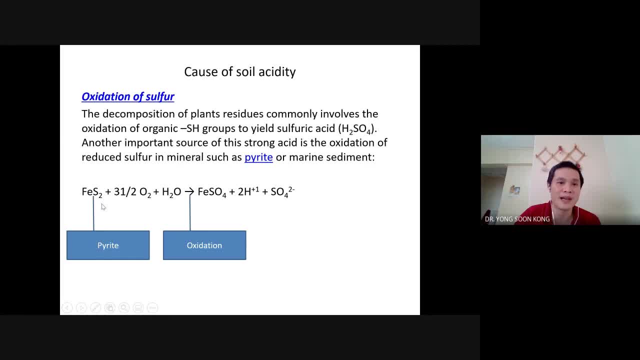 If you haven't seen pyrite before, this one looks exactly like gold, shiny yellowish. but it's not gold. It only contains iron and sulphide. So this is sulphide, you know, And this is all it takes to actually acidify the soil. 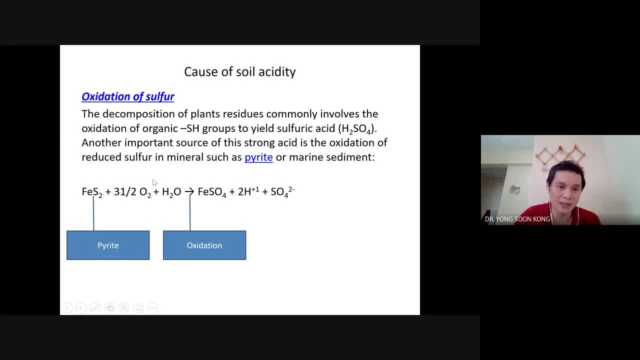 And once again, how does it happen? The oxygen in the atmosphere, It will oxidize the sulphur in pyrite And then it becomes sulphuric acid. Now you probably cannot see sulphuric acid because the sulphate already combined with. 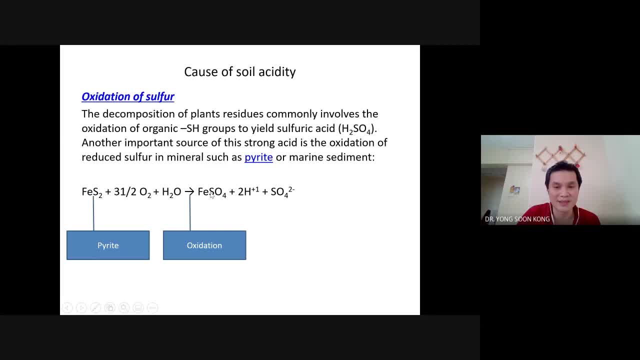 iron. So this is actually from the sulphuric acid. What you get is these two H+, And this is also one of the major reasons of soil acidification in a few parts in Malaysia. Now, the take home message is that If you have any sulphur element hanging around exposed to oxygen, it will become acid. 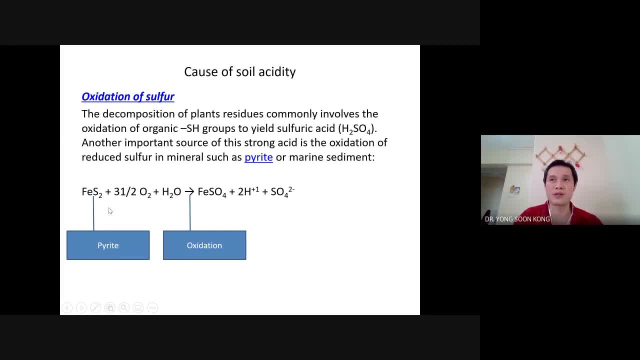 So it doesn't have to come from pyrite. It also can come from your belerang or sulphur powder, the yellowish colour ones. They also can do the same job. As long as you have sulphur element and oxygen, you will have sulphuric acid. 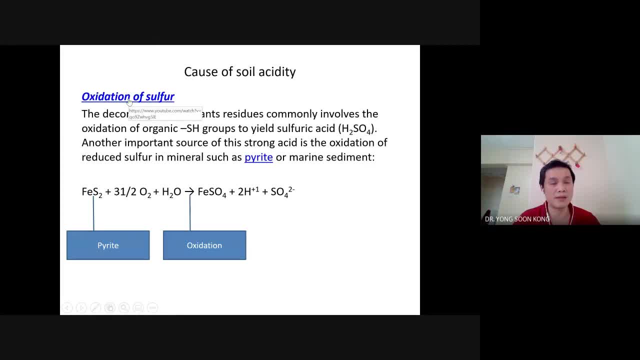 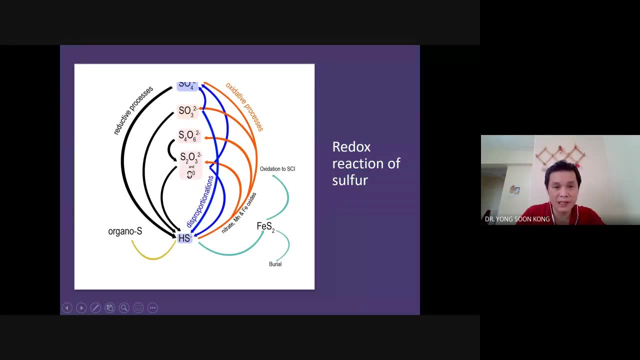 And once again, I think these are- yeah, these are- YouTube videos. So after this, go click it yourself and then watch the YouTube video on how sulphur can be oxidized to become acid, And this flow diagram shows you exactly how sulphur element from the center of this diagram. 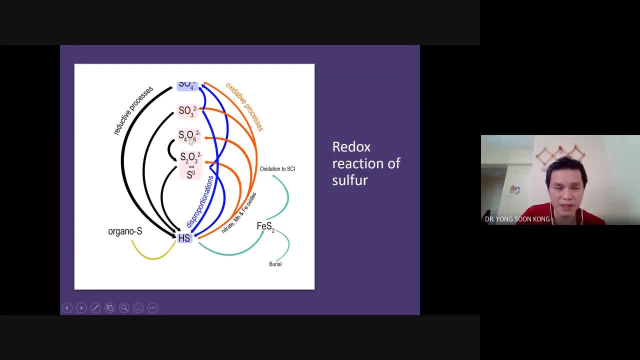 can be oxidized upwards. So if move up, if it moves up, it's slowly oxidized to become sulphuric acid. So this is the last destination. It becomes sulphuric acid and this is the strongest acid they can become. Okay, But at the same time, if you don't have enough oxygen, let's say this sulphur is buried deep in the soil, or maybe the soil moisture completely submerged the sulphur, it may become reduced, Because without oxygen it will be reduced and it becomes thiol. 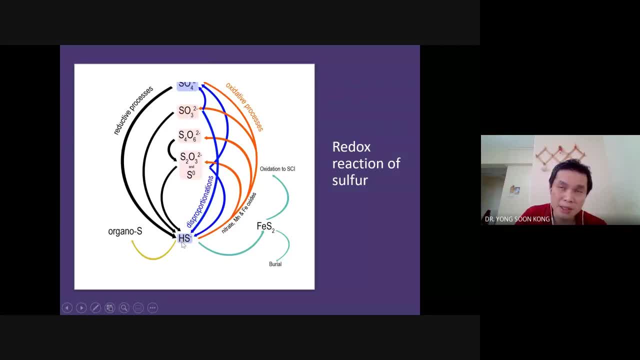 This is what we call it HSS, In other words, we call it thiol, so it becomes organosulphur, And this is the one that. This is the one that gives you the rotten egg smell. Yeah, this one, the rotten egg smell. 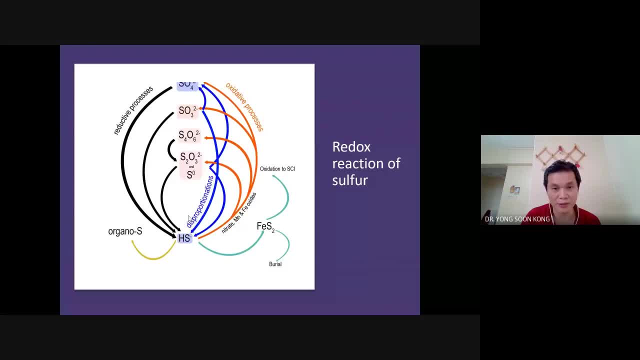 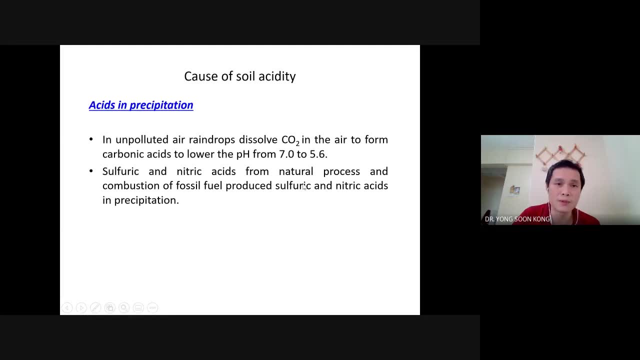 Yeah, a lot of chemistry. You can refer to that later on. And then what else? Yeah, the pollution. As I said to you just now, air pollution. If the air contains a little bit too much of nitrogen oxide or sulphur dioxide, it's. 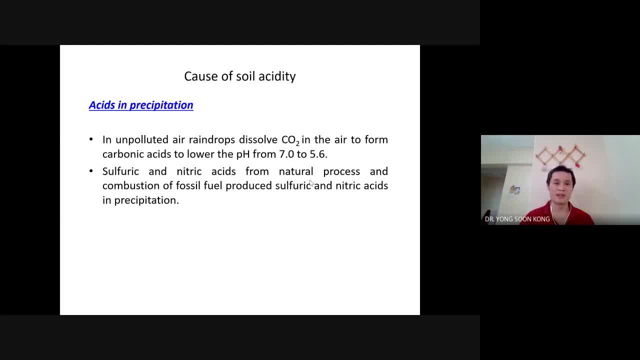 the same thing: You'll get more nitric acid, you'll get more sulphuric acid and therefore the pH of rainfall: it becomes acidic. Okay now, before I move on to the last cause of the acidity, actually in urban areas like 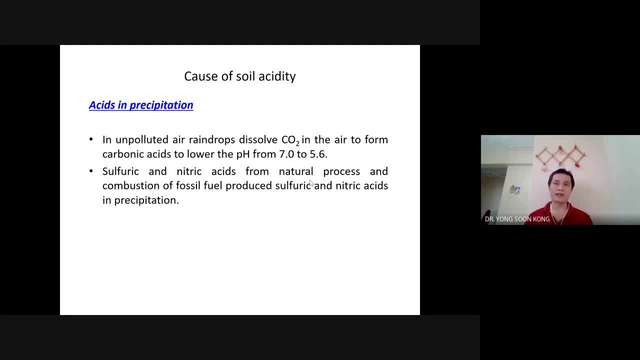 in Clang Valley, most of the soil in Clang Valley actually having a soil pH of 3 to 4. It's quite acidic Reason because of the cars and the factories that we have in the urban area. So that is a source of those nitrogen oxide and sulphur oxide. 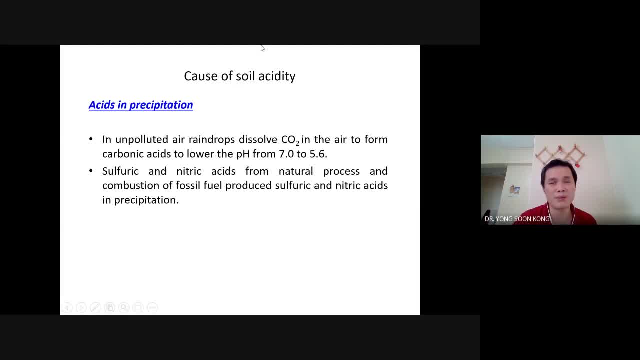 Therefore, when precipitation comes down, it brings all this acidity back to the soil and therefore the soil. for example, in PGA alone, maybe even Shah Alam also, the soil pH, if you say 4.5, that's quite normal, that's quite average actually. 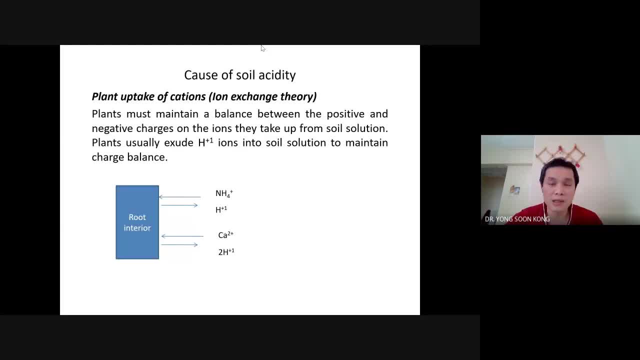 Okay now, moving on to the last cause, the last cause of soil acidity. you probably won't think of this, but it's natural. It's due to plant uptake. Okay Now, earlier I told you the presence of calcium cause soil to become alkaline. 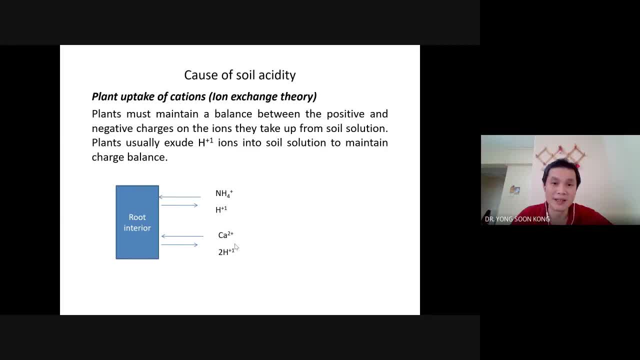 Without this cation, the soil becomes acidic, And this is precisely what the forests do. You see, forests actually have a lot of big trees And these trees exist for such a long time, So, in essence, these trees has been absorbing from the same spot. 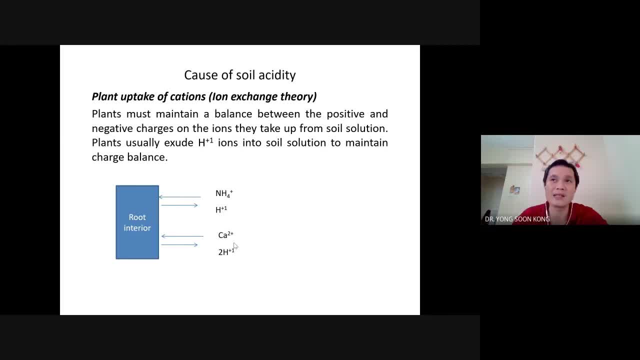 The same cations as its essential nutrient, And part of this nutrient, apart from ammonium, is also calcium, or calcium is the major source of mineral that gives you the alkalinity. Now imagine: one tree already exists in one same spot for the past hundreds or maybe thousands. 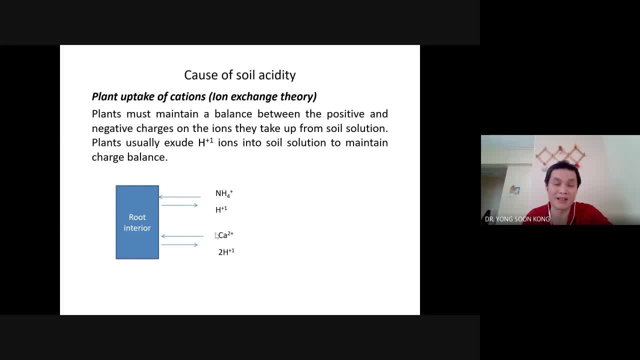 of years. Guess what happened to the soil? Yeah, it becomes acidic. Okay, So this is not due to human pollution. it's not due to pollution. By having uptake, extensive uptake, of these alkaline cations, the soil naturally becomes.